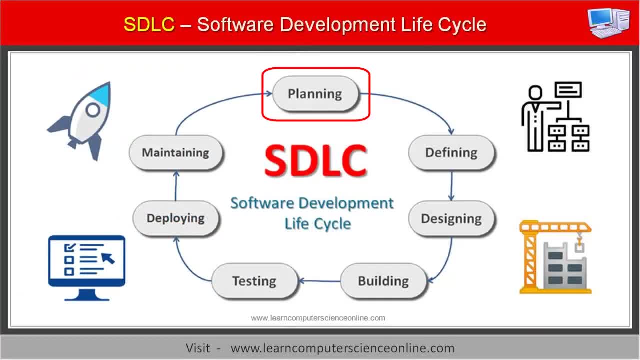 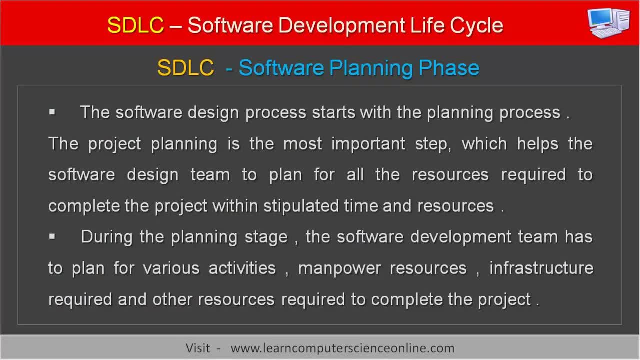 of these software design phase in detail. The software design process starts with the planning process. The planning process is the most important step, which helps the software design team to plan for all the resources required to complete the project within stipulated time and resources. 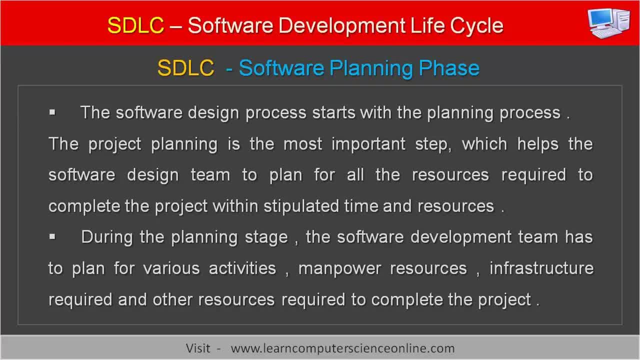 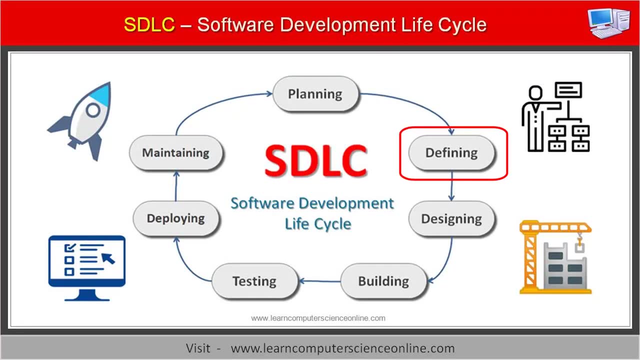 During the planning stage, the software development team has to plan for various activities: manpower resources, infrastructure required and other resources required to complete the project. The next phase in the software development process is referred to as defining the software requirements. This process is also alternately referred to as requirement solicitation. 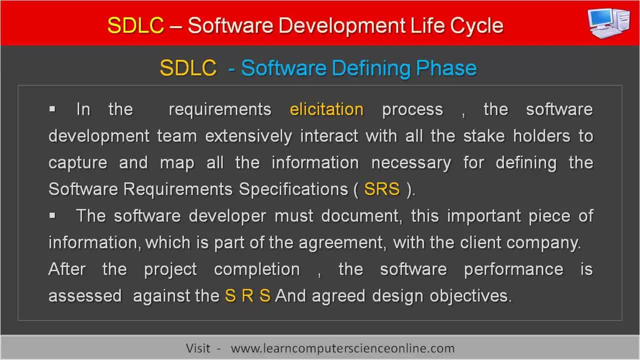 In the requirement solicitation process. the software development team extensively interact with all the stakeholders to capture and map all the information necessary for defining the software requirements specifications. These user requirements document is abbreviated. The software developer must document this important piece of information which is part of the agreement with the client company. 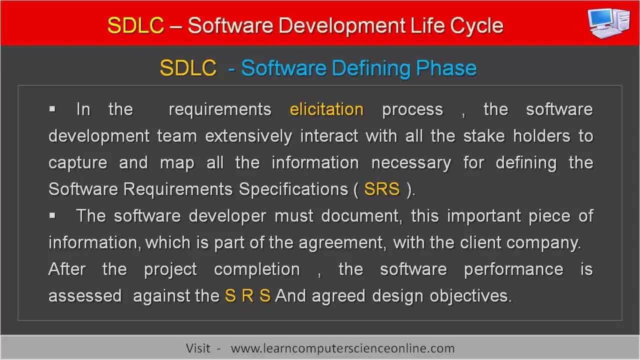 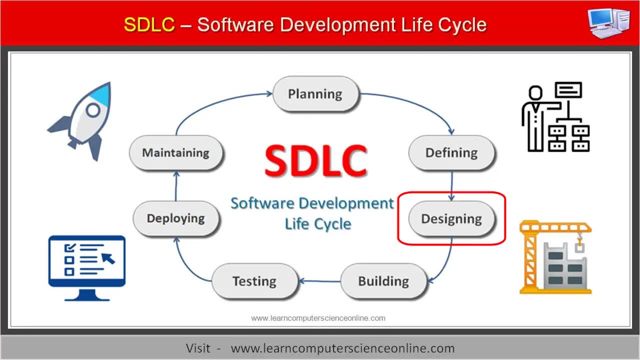 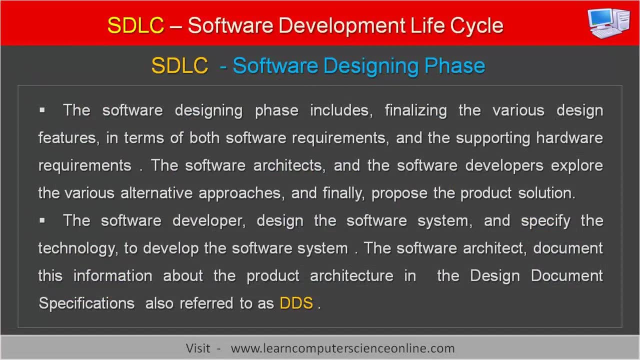 After the project completion, the software performance is assessed against the SRS and agreed design objectives. The next and third phase in the software development process is referred as designing the software. The software designing phase includes finalizing the various design requirements. 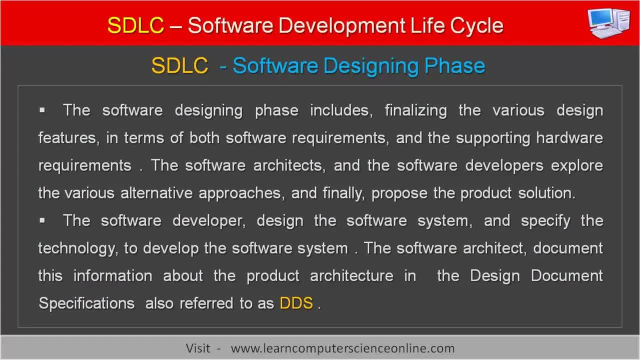 The software design features in terms of both software requirements and the supporting hardware requirements. The software architects and the software developers explore the various alternative approaches and finally propose the product solution. The software developer design the software system and specify the technology to develop the software system. 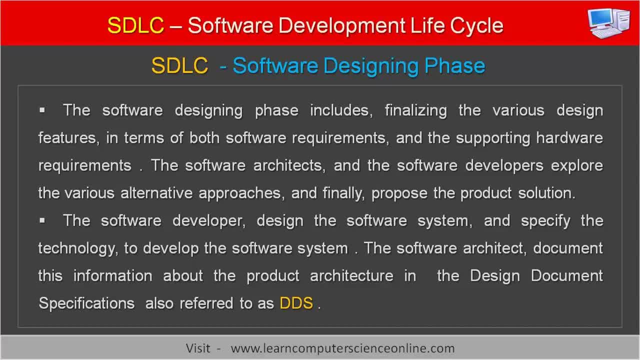 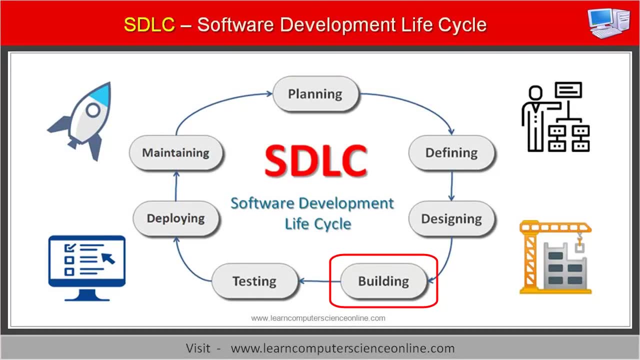 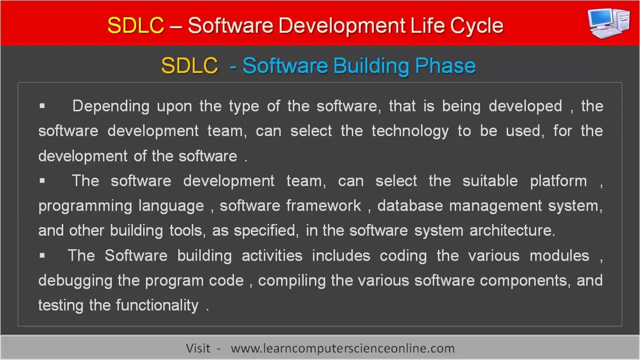 The software architect document. this information about the product architecture In the design document specifications, also referred to as DDS. The next and fourth phase in the software development process is actually building the software with suitable technology and tools, After finalizing the software requirements, specifications, SRS, software design features and the software system architecture. 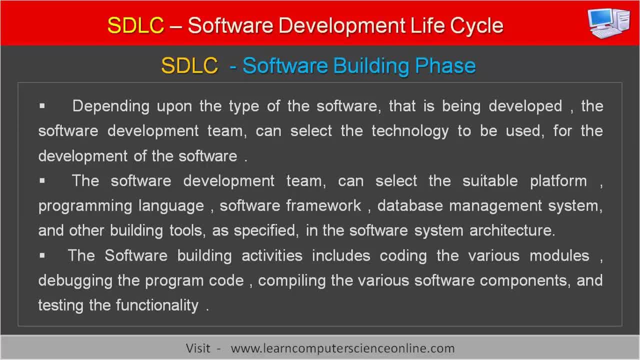 The next step is to actually start building the software by coding. Depending upon the type of the software that is being developed, the software development team can select the technology to be used for the development of the software. The software development team can select the suitable platform, programming language, software framework, database management system and other building tools, as specified in the software system architecture. 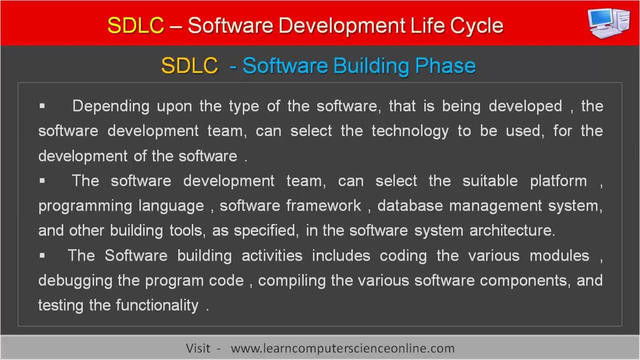 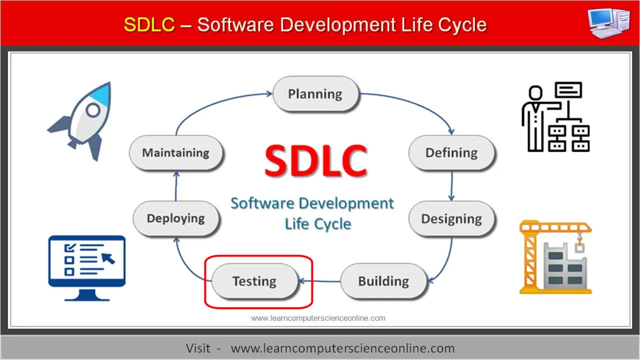 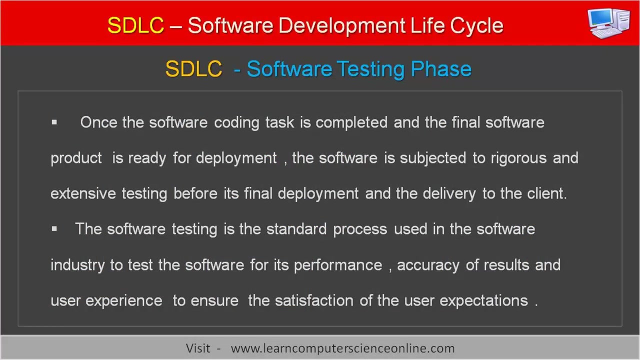 The software building activities includes coding the various modules, debugging the program code, compiling the various software components and testing the functionality. The next and fifth phase in the software development process is the software testing. Once the software coding task is completed and the final software product is ready for deployment, the software is subjected to rigorous and extensive testing before its final deployment. 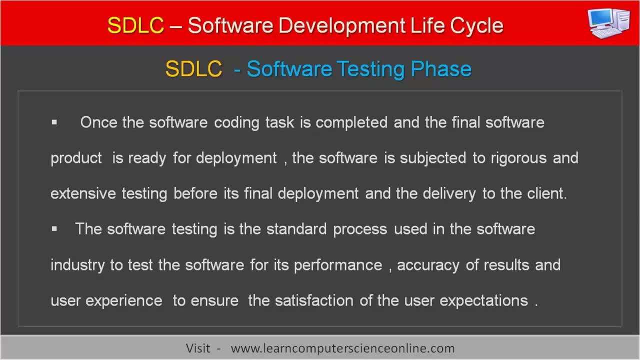 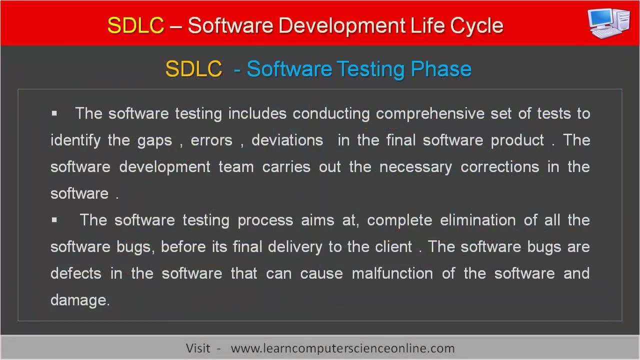 And delivery to the client. The software testing is the standard process used in the software industry to test the software for its performance, accuracy of results, user experience. to ensure the satisfaction of the user expectations, The software testing includes conducting comprehensive set of tests to identify the gaps, errors, deviations in the final software product. 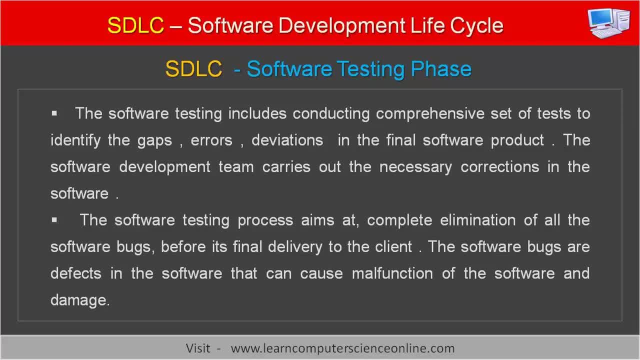 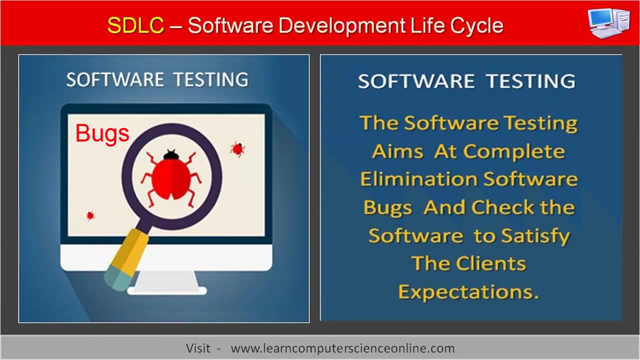 The software development team carries out the necessary corrections in the software. The software testing process aims at complete elimination of all the software bugs before its final delivery to the client. The software bugs are defects in the software that can cause malfunction of the software and damage. 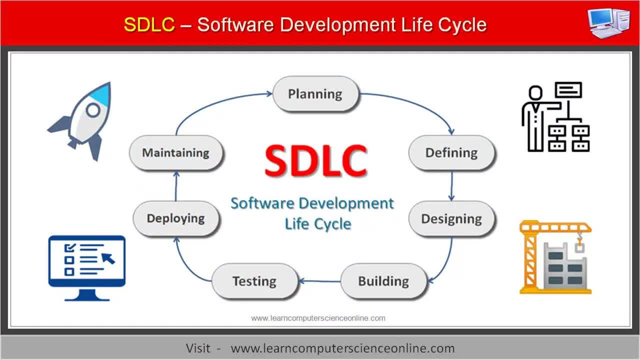 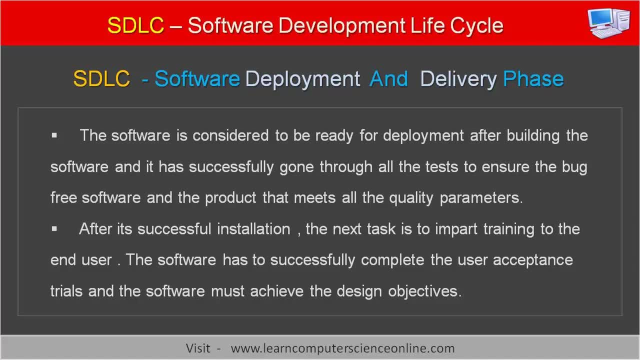 The next and sixth phase in the software development process is the software deployment and its successful installation. The software is considered to be ready for deployment after building the software and it has successfully gone through all the tests to ensure a bug free software and other quality parameters. 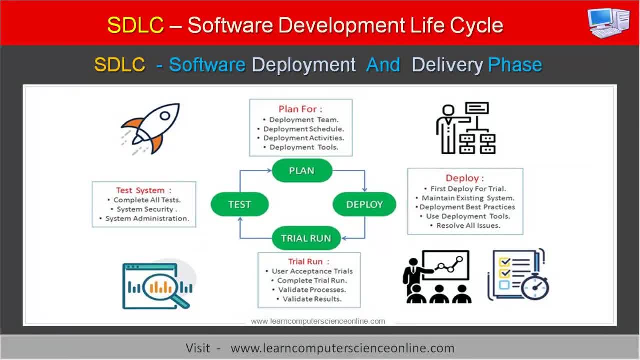 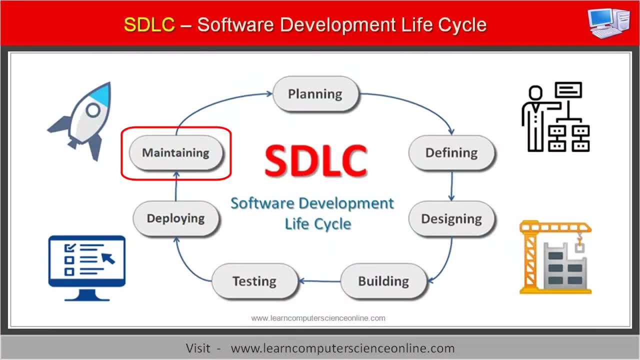 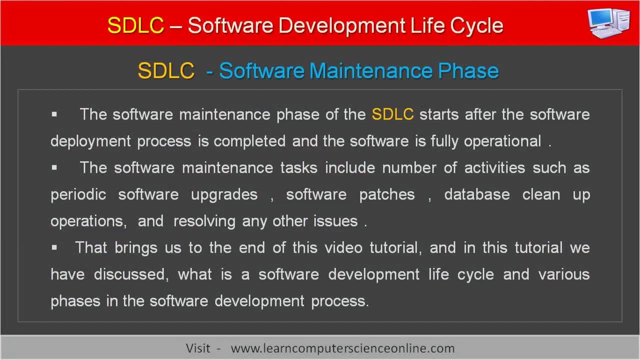 After its successful installation, the next task is to impart training to the end user. The software has to complete user acceptance trials. The last and seventh phase in the software development process is the software maintenance phase. The software maintenance phase of the SDLC starts after the software deployment process is completed and the software is fully operational.